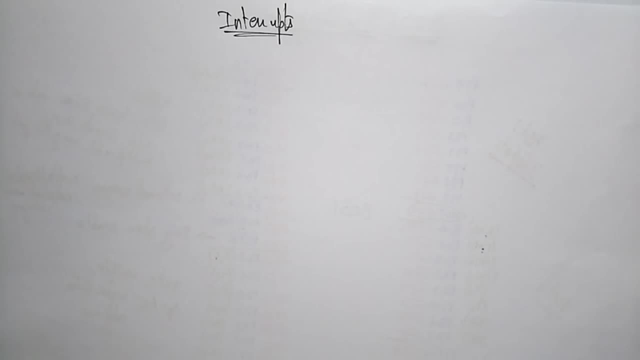 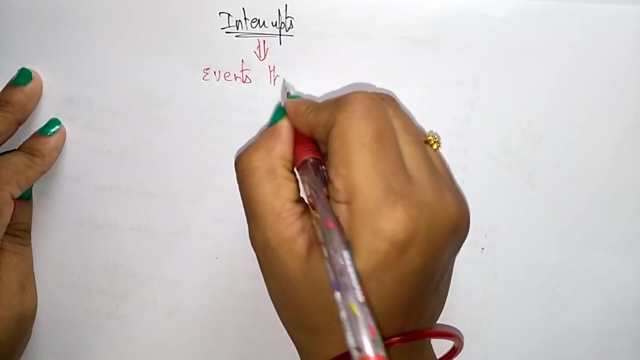 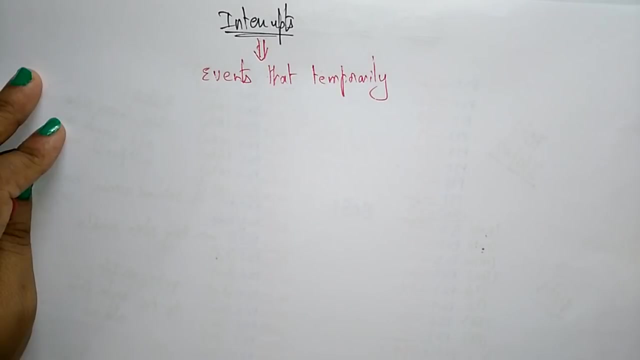 Hi students, welcome back. Coming to the next topic, that is, the interrupts. So what is an interrupt? So everyone will know that interrupts are the events. We just call it as an events that temporarily suspends the main program. So I already explained about this interrupt. Let me write again: Interrupts are nothing but events that temporarily suspend the main program. 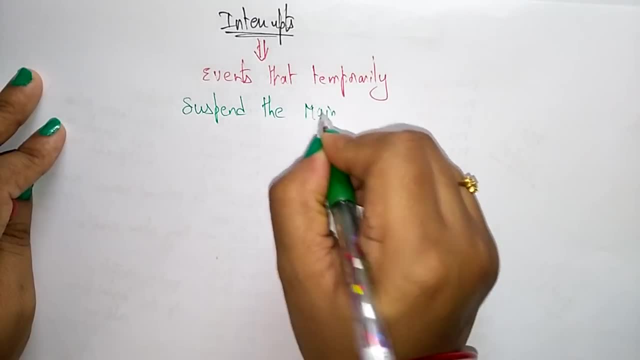 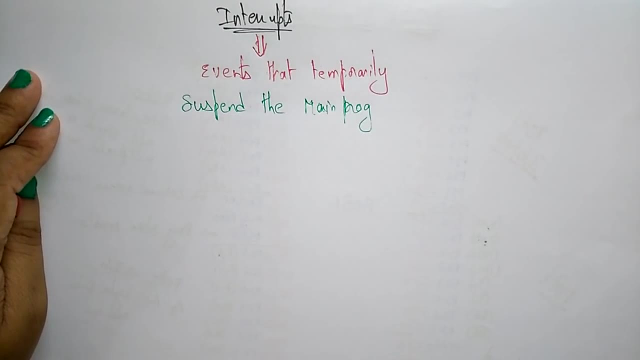 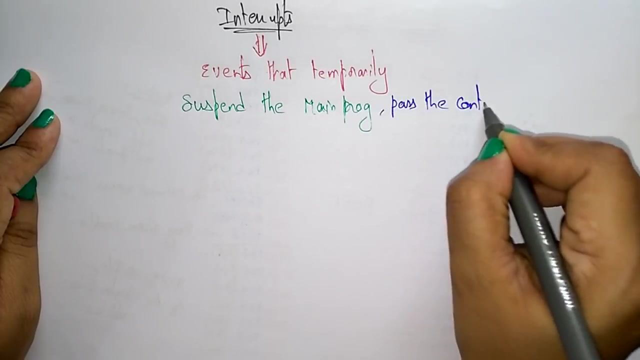 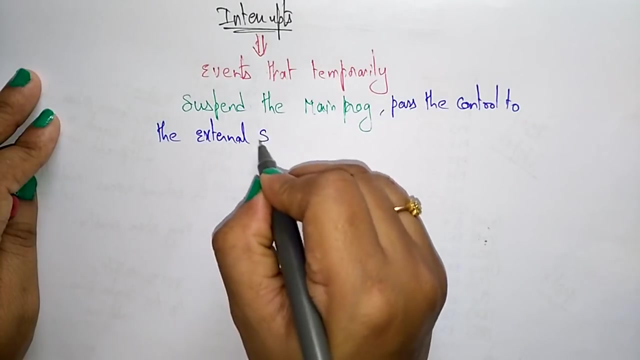 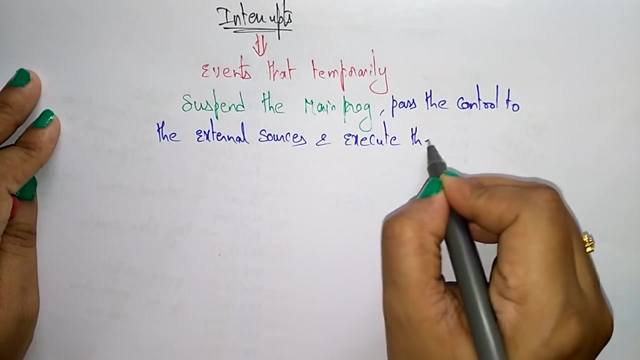 So, whatever the professor is doing, operation means the main program, so that will be suspended. Interrupts are the events. Interrupts are the events, events that temporarily suspend the main program and pass the control to and pass the control to the external sources, external sources- and execute the task and execute the external. 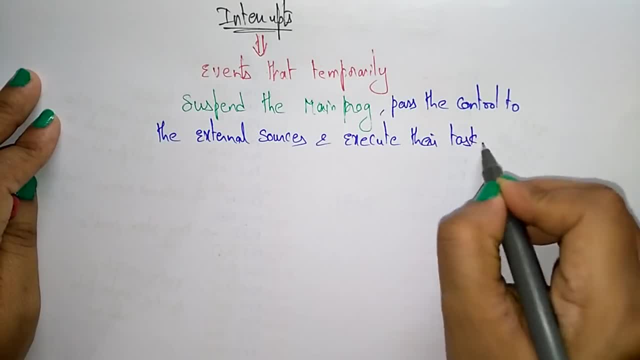 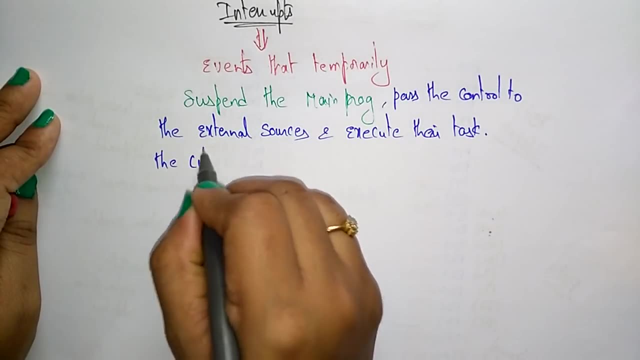 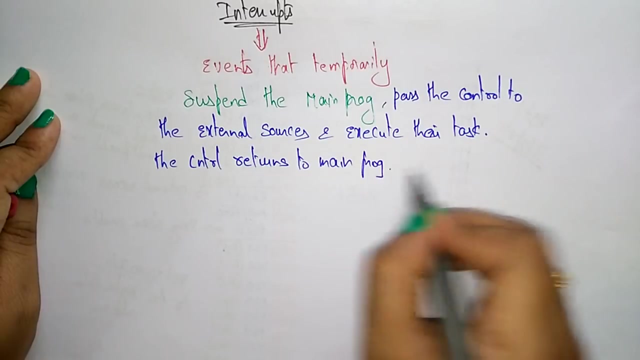 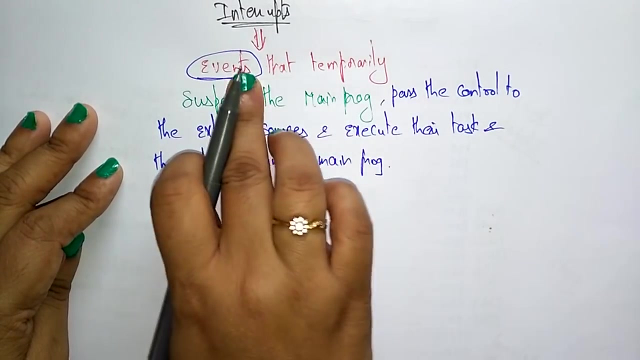 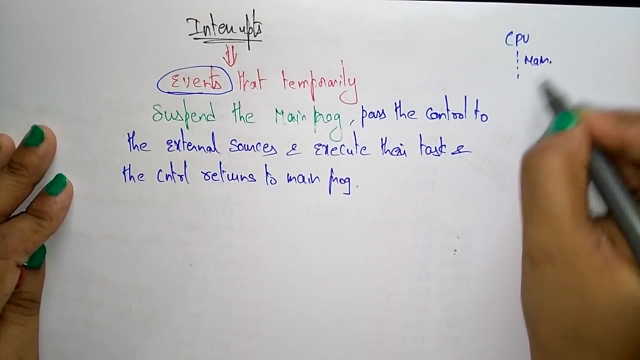 source task execute their task. okay, so after completion of the task, the control returns to main program. the control returns to main program. okay, so that is an interrupt. so interrupts are nothing but event events that temporarily suspend the main program. so whatever the CPU is doing, uh, accessing main program, suddenly interrupt occurs. okay, the signal will transmit to that. 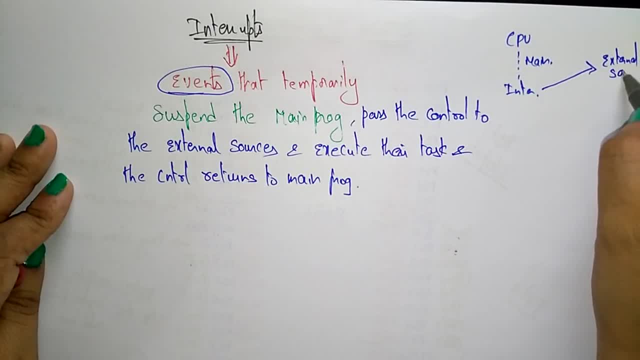 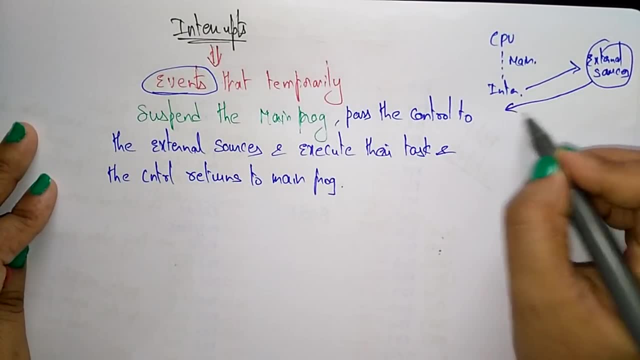 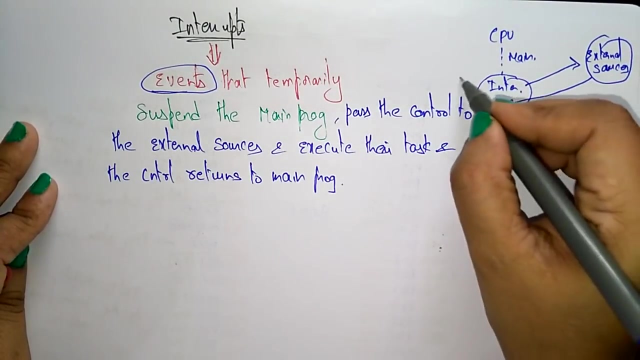 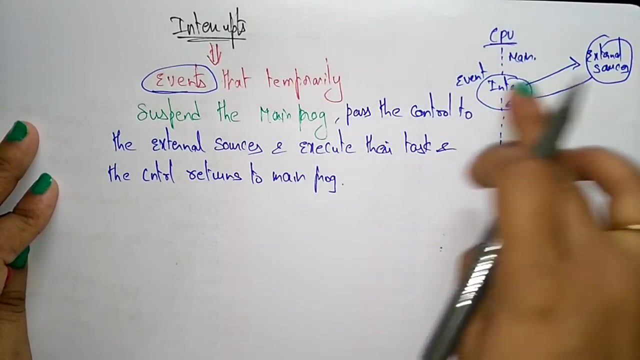 external sources: external sources. after completion of the external sources, execution again the control transmit, return back to the main program and continue with the program. okay, so this is a nothing, but it is an event, okay, whenever the CPU is doing some um uh, executing some uh, coffir地, anything event happen when you have a 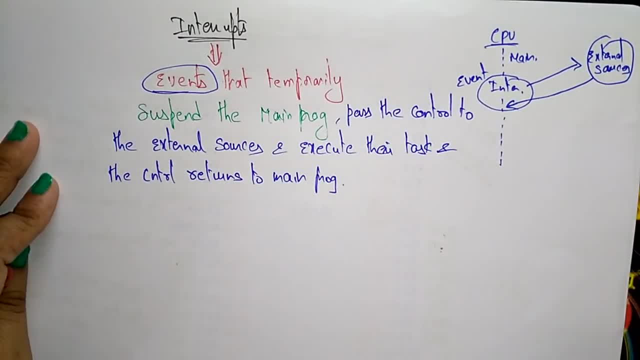 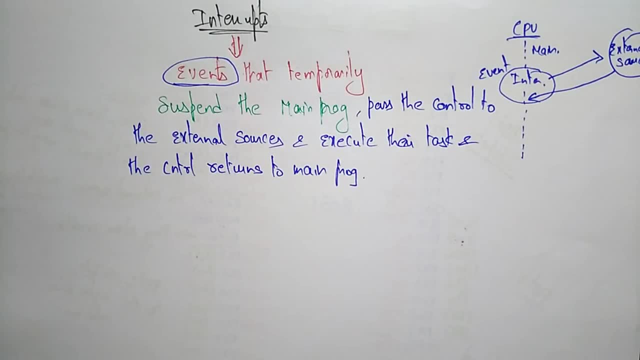 karters, because they used to have the main program. whenever the event is occurred, the control transferred to the external resources and execute the task and return back to the main program. that you call it as inter interrupts is nothing but a disturbance. caused it to cpu? okay, suppose if I am teaching something suddenly phone calls came to me then that. becomes an interrupt to me. okay, that phone call is uh halting my, uh, my recording. okay, and uh, i want to answer the fact and I'm getting another call when I'm doing another call and I'm in it again, as you can see, uh, which of the different uh uhhols handbook and volume. 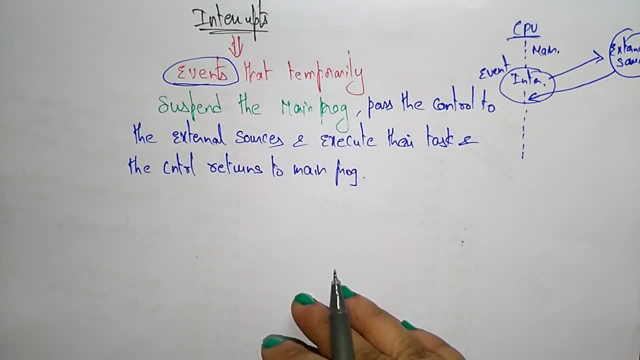 scanner very strong, right, is it? that is helpful to enjoy that. okay, if you can apply to the participation And I want to answer that call After the completion of the. after answering the call, I again continue my recording. So that is an interrupt. 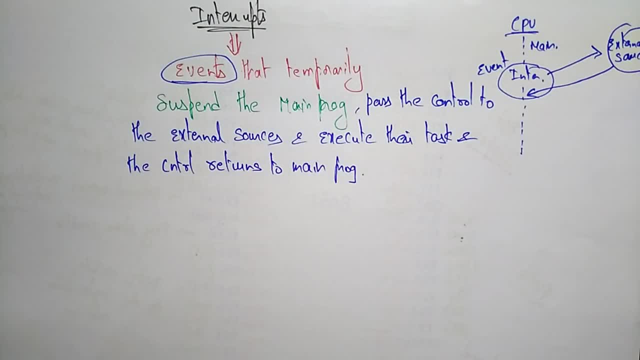 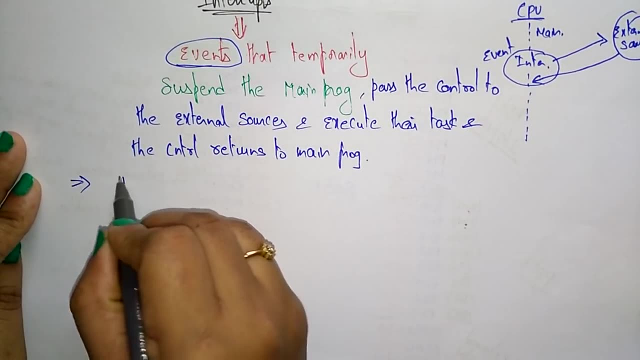 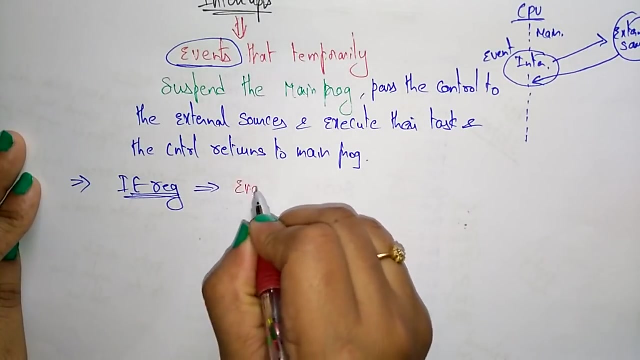 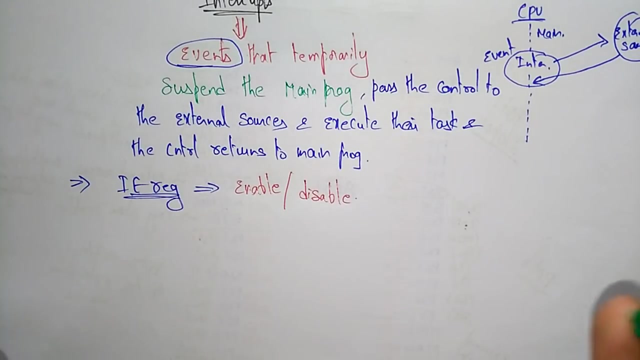 So if anyone anything is disturbing me that we call it as an interrupt, So here each interrupt can be enabled or disabled by using IE register. So with the help of IE register the interrupt can be enabled or disabled And the whole interrupt system can be disabled by clearing EA bits of same register. 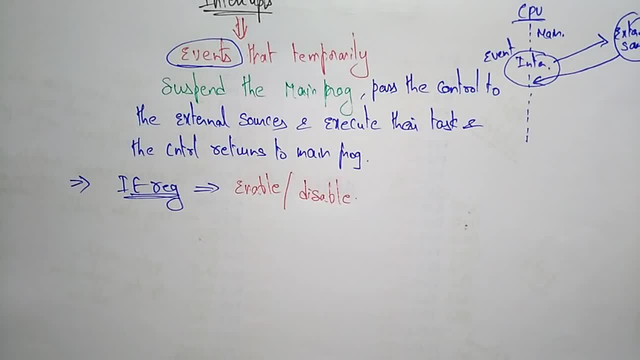 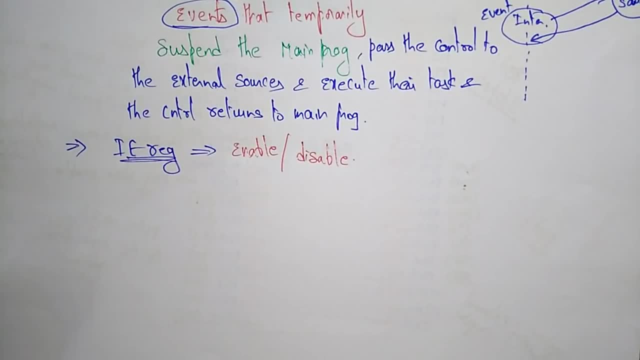 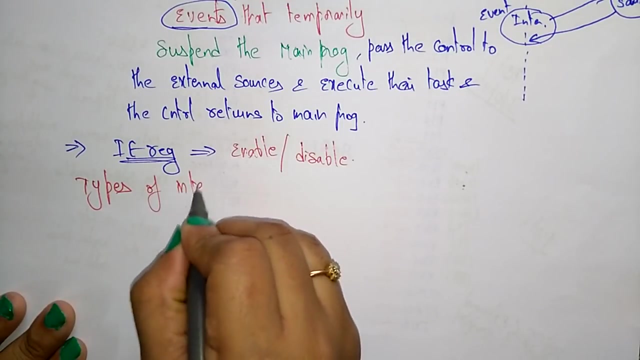 It means external access bits has to be cleared Whenever this interrupt system can be disabled by clearing EA bits of same register. Let me write the different types of interrupts that are present in 8051 microcontroller. Types of interrupts in 8051 microcontroller. 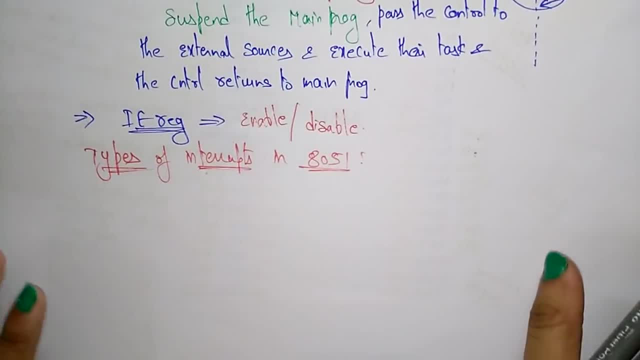 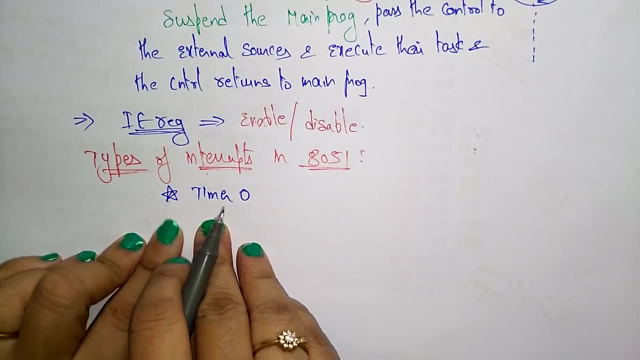 So what are the different types of interrupts that are present here? First one, timer 0.. So timer 0 is one of the interrupts that cause it to the 8051 microcontroller, which we call it as a overflow interrupt. 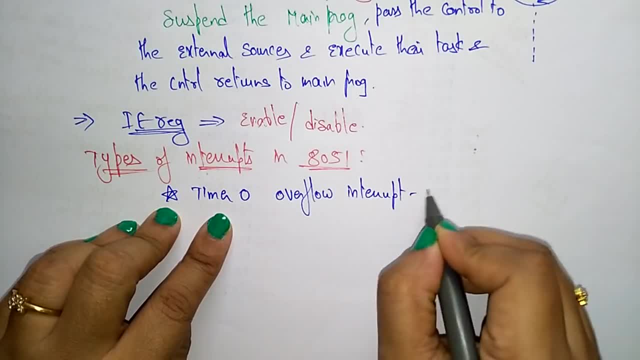 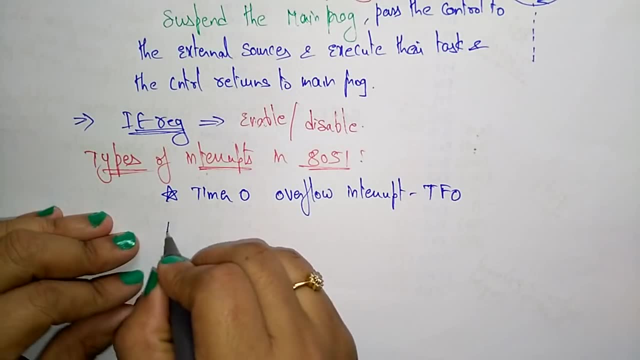 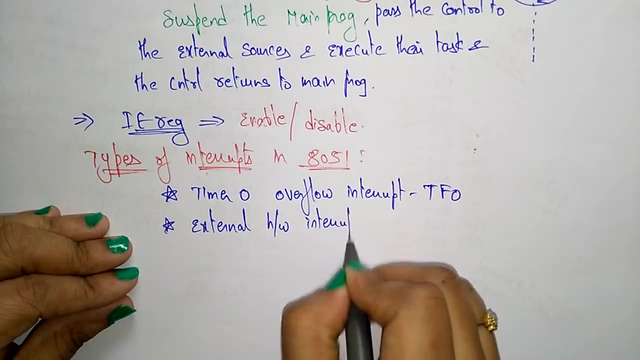 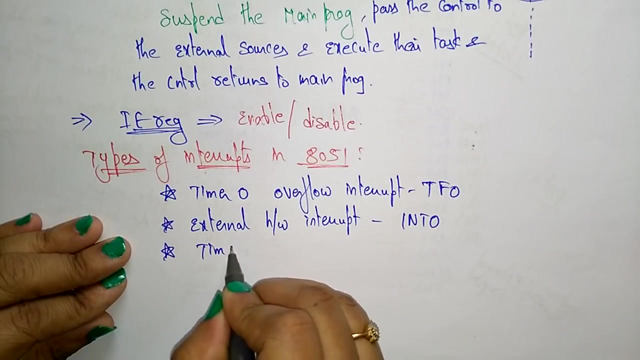 Overflow interrupt So that TF0.. So whenever the TF0 is nothing but it is a timer 0 overflow interrupt. And next, external External hardware interrupt. External hardware interrupt is INT0.. And next, timer 1 overflow interrupt. 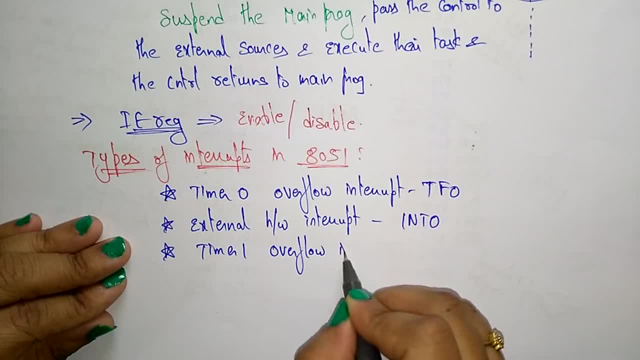 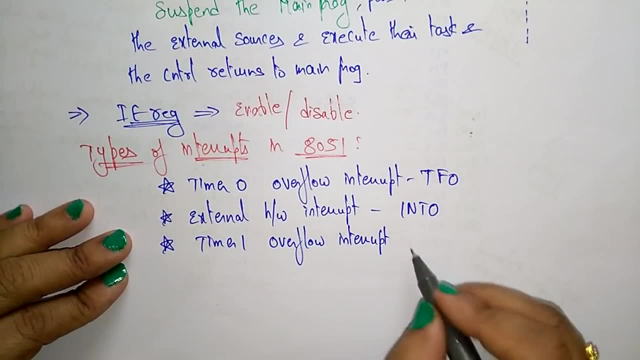 Timer 1: overflow- interrupt. Actually, two timers will be there: Timer 1 and the timer 2.. That 16 bit will be divided into two, 8 bits, So timer 0 and the timer 1. That is timer F1.. 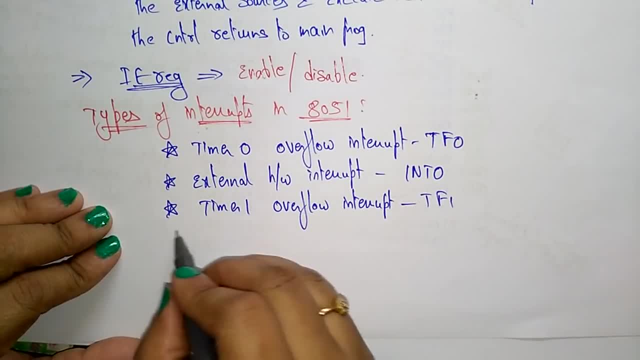 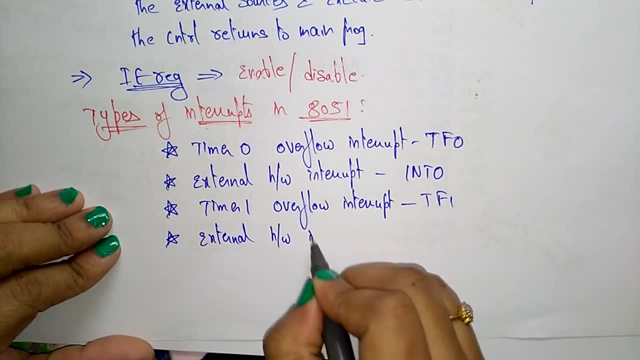 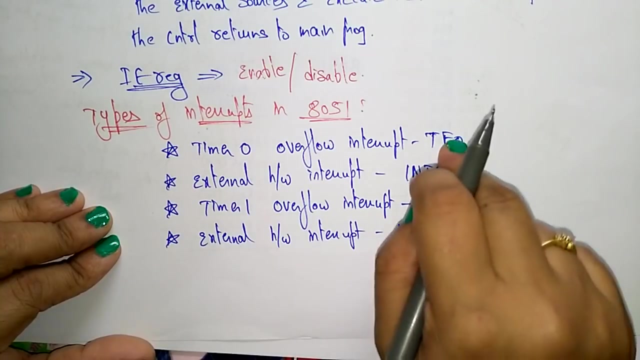 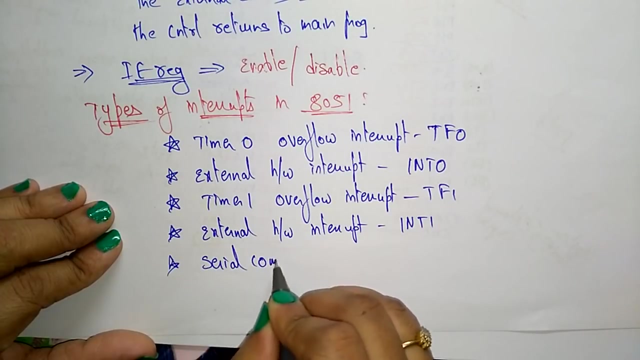 Timer. F1. overflow interrupt And external hardware interrupt. you are again having External hardware interrupt, INT1.. So INT1, TF1.. INT0, TF0.. And the next is a serial communication. interrupts will be there. Serial communication interrupt. 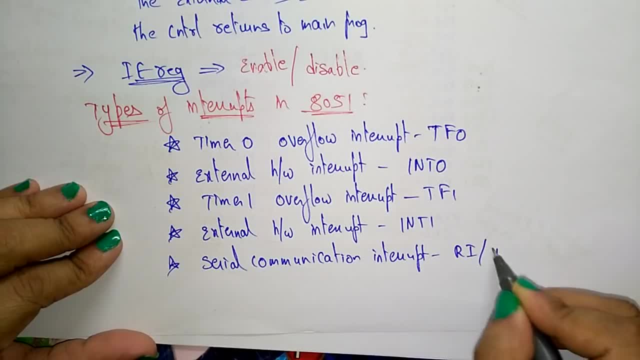 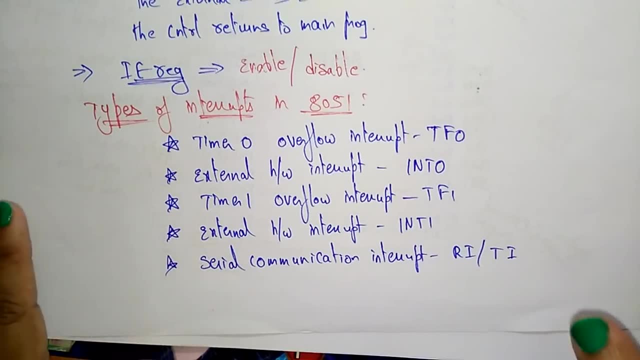 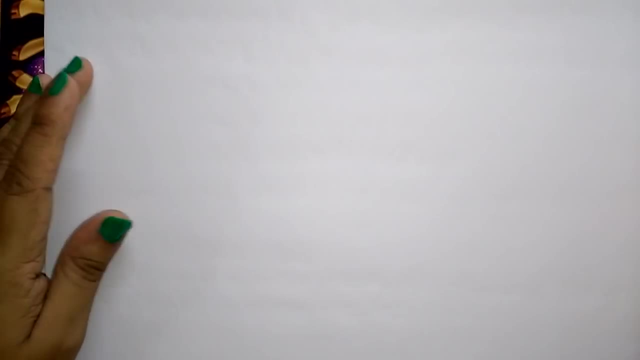 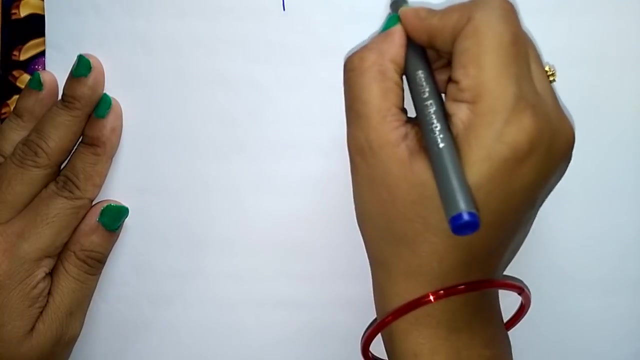 That is, RI and TF: Receive, interrupt and transmit interrupts. So these are the different types of interrupts that are present in 8051 microcontroller And let me explain some. interrupt vector table, Interrupt vector table. So this interrupt vector table. 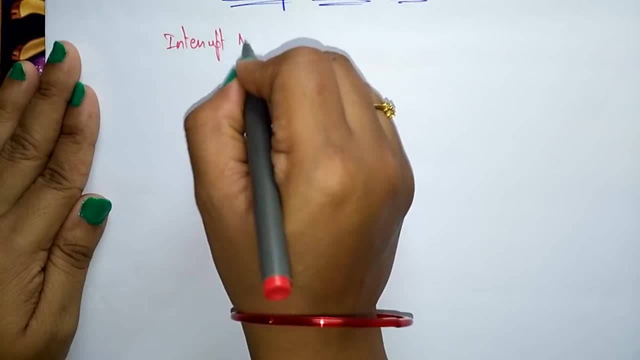 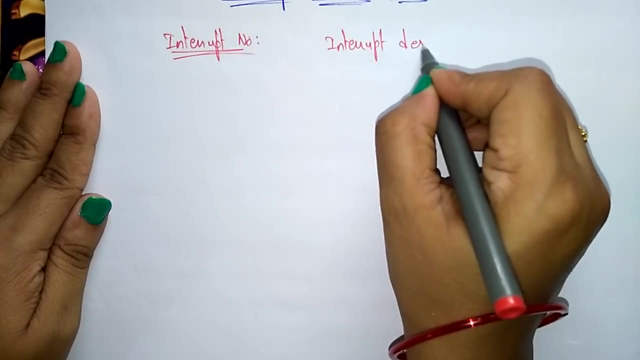 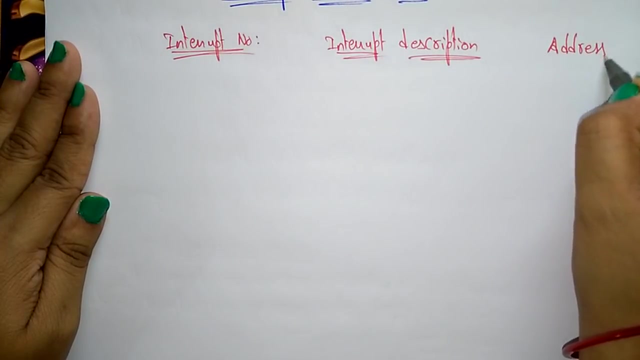 Let me write the interrupt number. So each interrupt They are having one interrupt number. And let me write the interrupt, That interrupt description, And then the address in which location this interrupt will be stored. Okay, And the address. So let us take interrupt 0.. 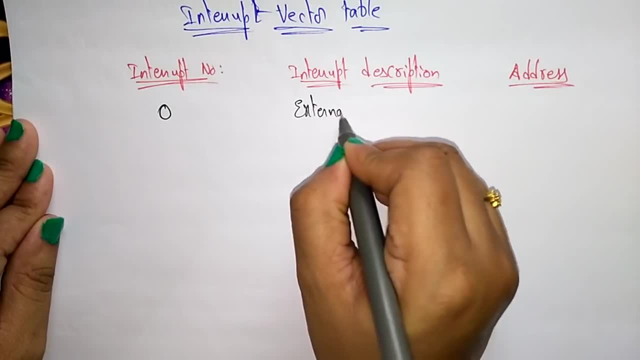 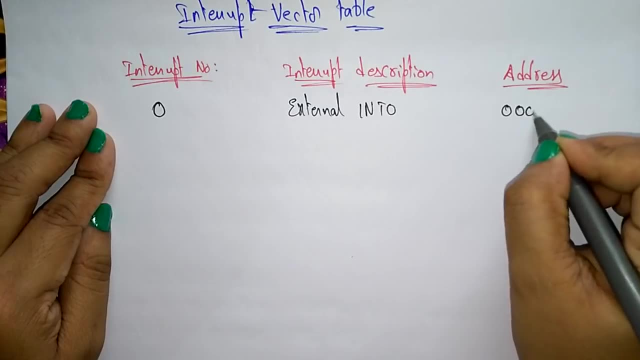 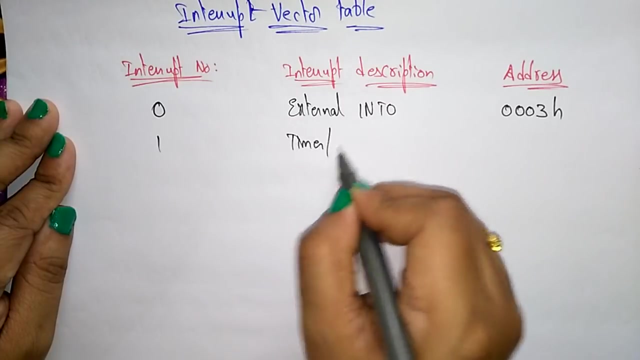 Interrupt 0 is nothing but external INT0.. So whenever the interrupt number is 0, it is nothing but external INT0.. And the address location is 0003H. hexadecimal Interrupt 1.. This may be a timer or counter 0.. 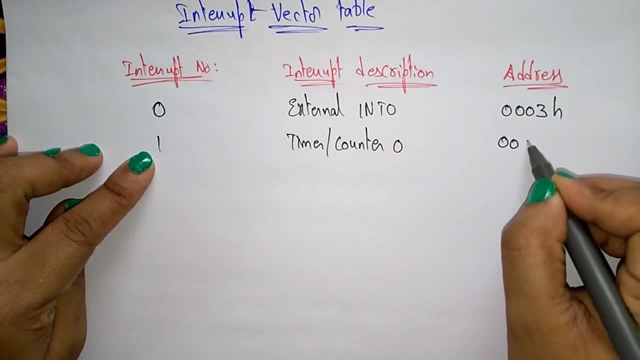 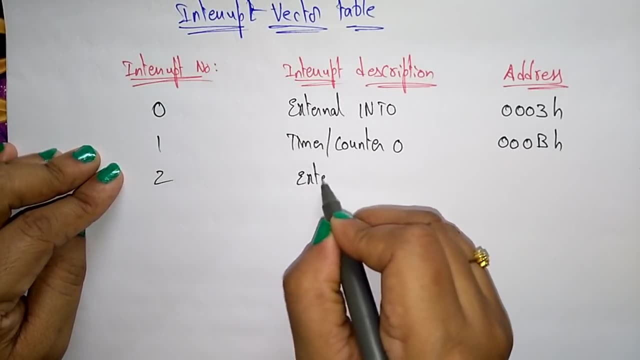 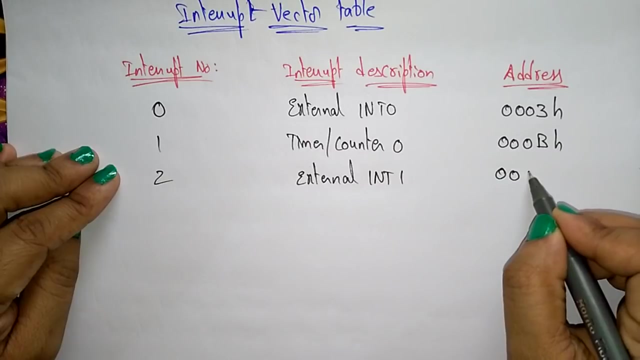 It may 1,. it represents a timer or counter 0.. And thus address location is 000BH. Next, 2. External interrupt: 1. INT1.. The address location is 00.. 1,, 3, H. 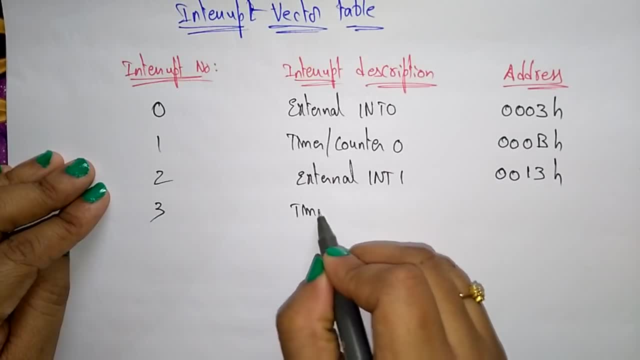 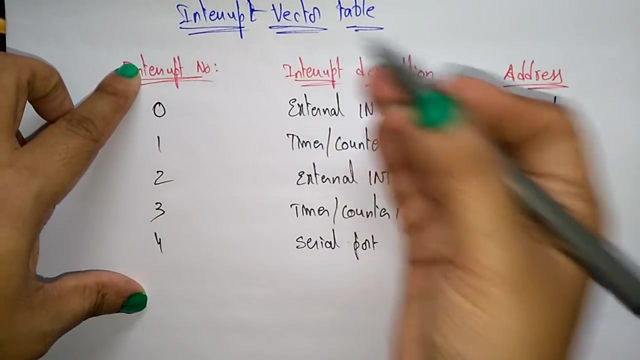 And 3. Again, the timer and counter. 1. 001BH And the 4th Serial port. So the different types of interrupt are represented in the form of vector table. So vector table indicates the address. A table indicates address. 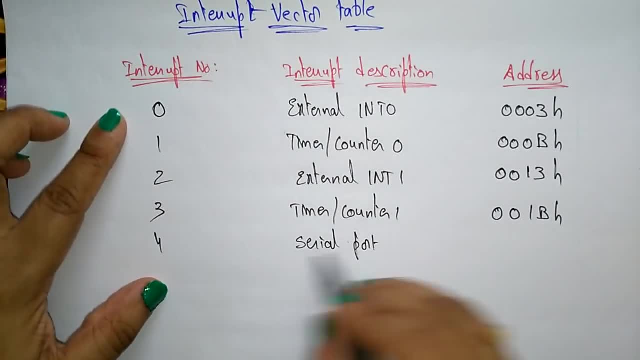 So in this particular address only those interrupts will be stored And the 4th In serial port vector Interrupt vector table address is 0023H. So this is about the interrupt vector table. So in the next video I will explain about the interrupt enable and the interrupt priority registers.